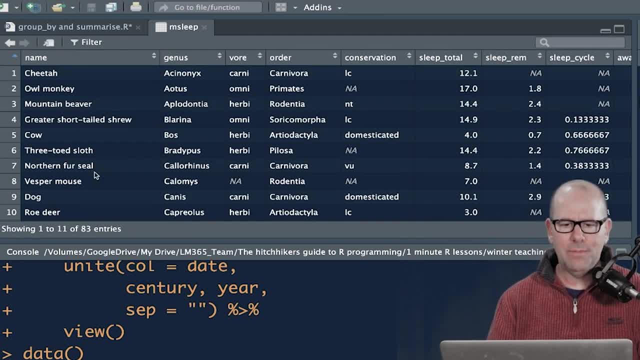 mammal sleep, right. We've got all of our mammals here: cheetahs, lions, blah, blah, blah, blah. And then they're categorized by omnivores, herbivores, et cetera, et cetera. And then we've 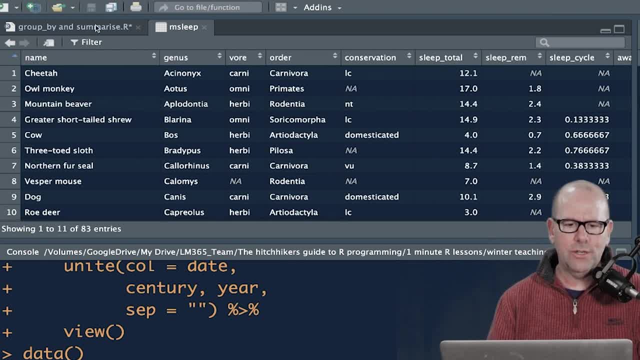 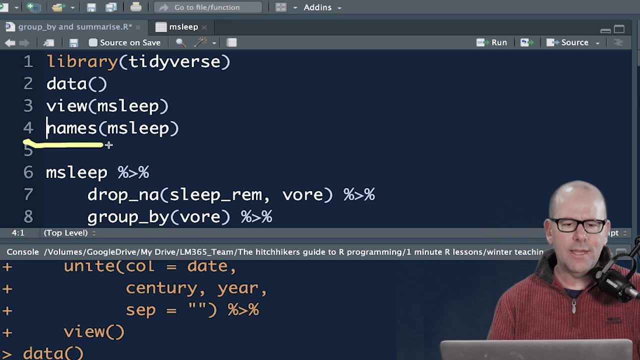 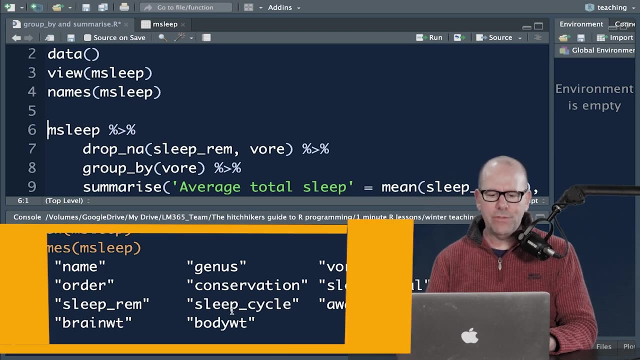 got characteristics of their sleep right there, So we're going to look at some of this today. I'll show you the data set. Names is quite a nice little function because you can just ask R to show you what, and I often use names because then all of the names of the variables pop up- What I like. 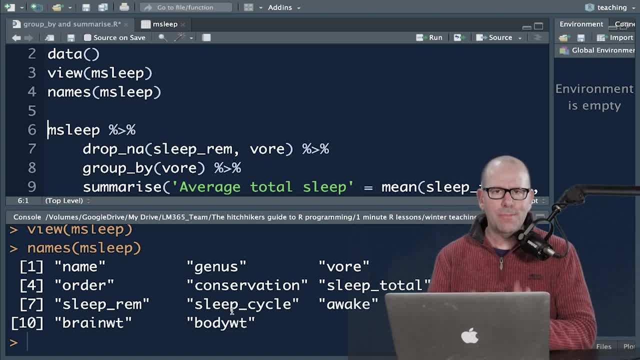 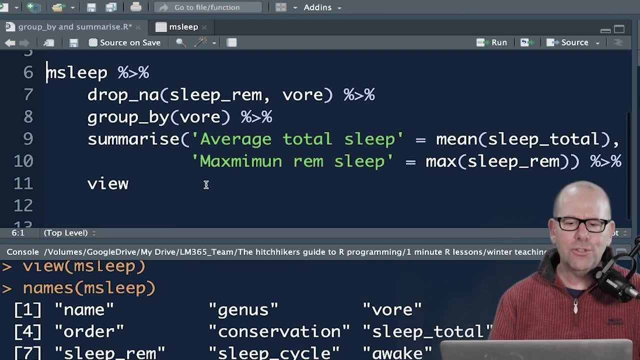 about that is I can cut and paste them into my code so I don't make spelling mistakes, Because one of the biggest problems when you're writing code is you kind of misspelled something, So I'll just cut and paste them straight from there. Let's look at the code for group by and summarize: 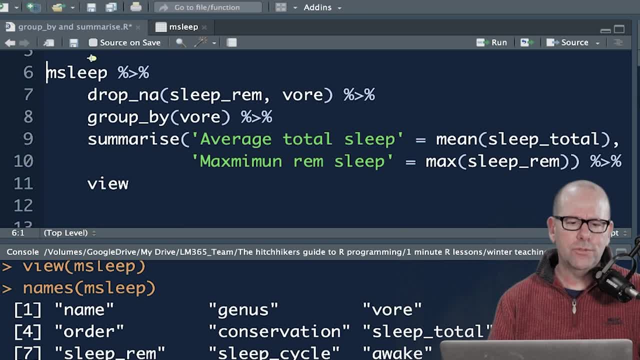 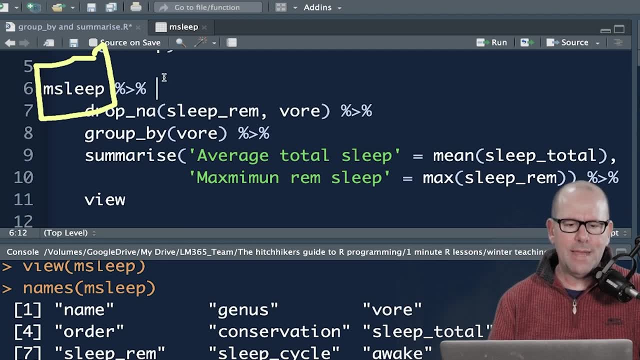 We start off. when we're working in the tinyverse, Your starting point is your data object. In this case it's the data set called m sleep, Whoops, Okay, Go back there. All right, Okay. Next thing is this pipe operator right, And that simply means and then So we're piping this data object. 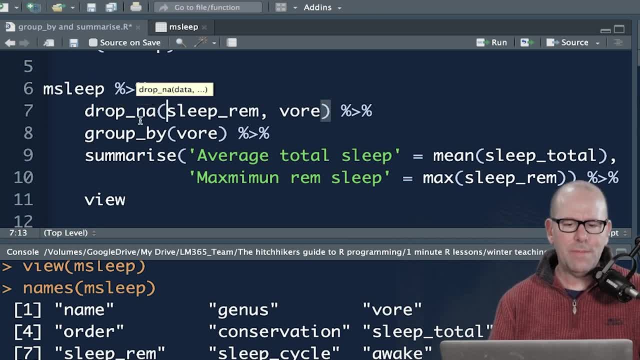 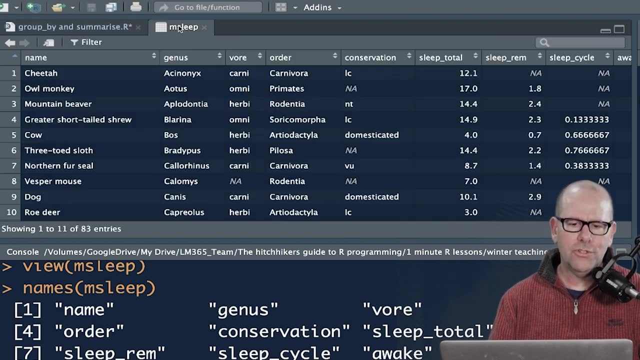 into the next line of code And this: drop na. I'm basically just going to remove missing values. Na is not available, So drop na. I'm removing missing variables from the sleep rem variable and from the vor variable, And I'll just show you what I'm going to be doing here. 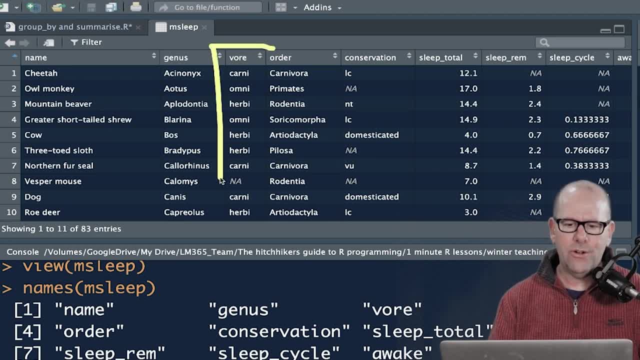 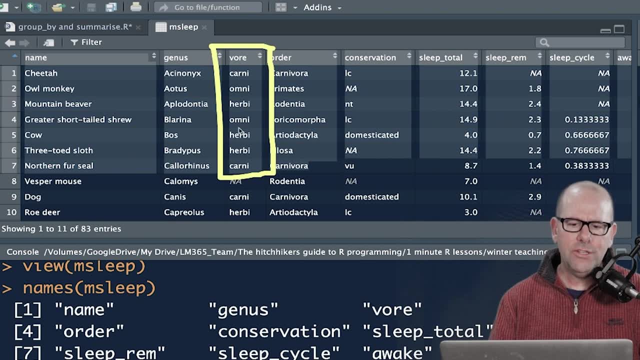 Looking at this variable here, vor, It's a categorical variable. That's going to be quite important when we talk about group by. Okay, And I'm going to ask R to take each of these categories and look at another variable. Okay, So we could take rem. sleep over here. 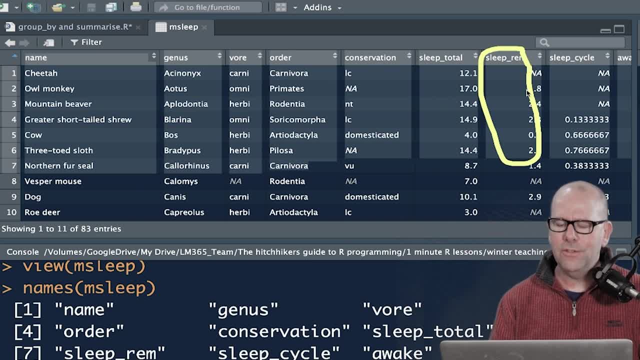 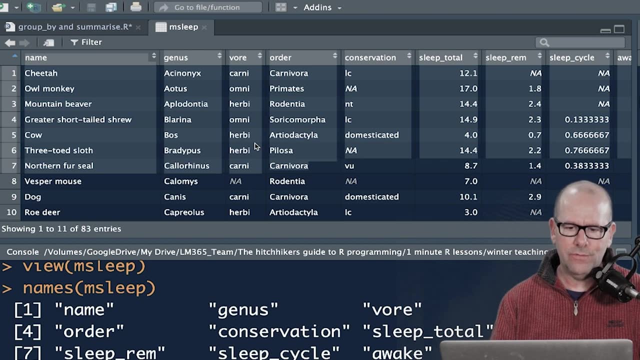 My drawing is terrible. I've crossed out half of the values. You know you get what I mean. And we are going to summarize these characteristics, characteristics of this variable, to what categories various observations land up within with respect to this categorical variable. 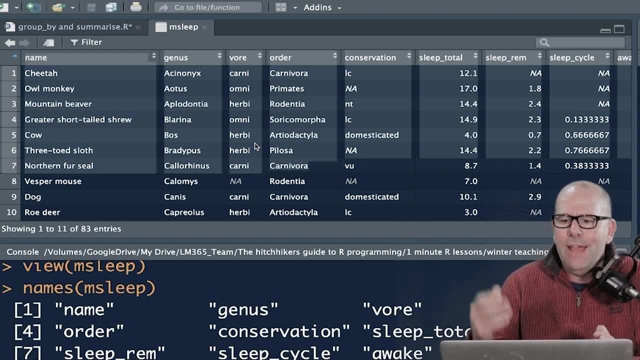 In other words, we'll take all of the carnivores and work out the average rem sleep, for example, and all of the omnivores, work out the average rem sleep for them, etc. etc. But it's no good if there's missing values, particularly with respect to the rem sleep, Because if there are, 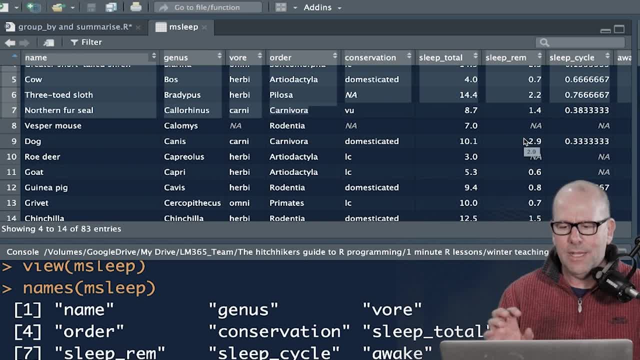 missing values. it's difficult to work out averages and stuff And you might have to like include omit na's into your code. it's easier. But for the sake of this, for the sake of this particular tutorial, is just to delete all the. 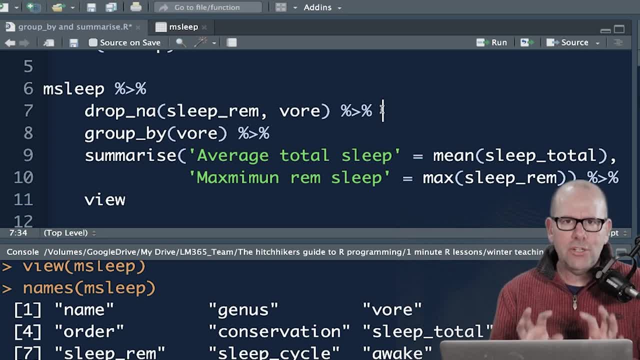 missing values right in the beginning. when you're dealing with missing values and you're actually analyzing your data, It's not good practice just to have a blanket remove all the missing values at the beginning And that's that. you really need to think about why values are missing. Okay, and 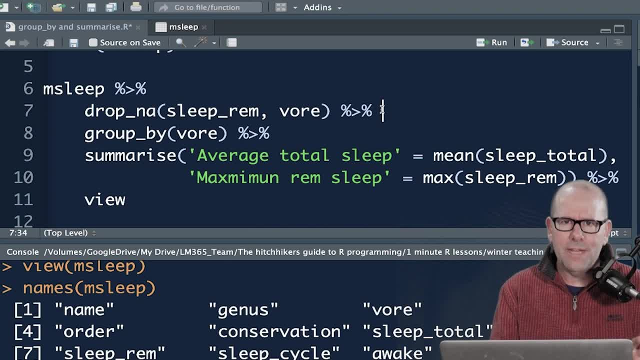 and remove missing values when it's appropriate, And I've got a video that talks all about missing values, So go and watch that if you find it confusing. But for the sake of this tutorial, we're going to drop the missing values from those two variables, right? 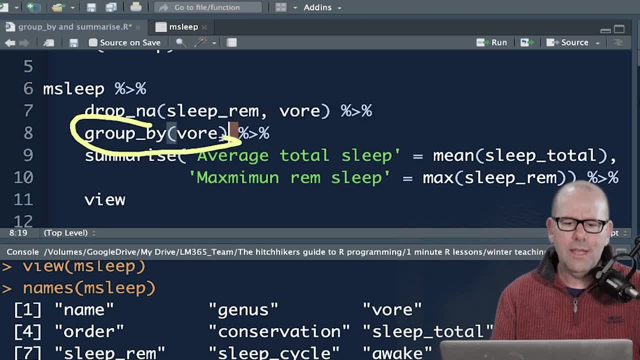 And that's where things get interesting, right. Group by- okay, we're grouping by a variable for, and then we're piping that in and then into the summarize function, And here the summarize function is going to create some new variable headings, right, And they'll be whatever you want. 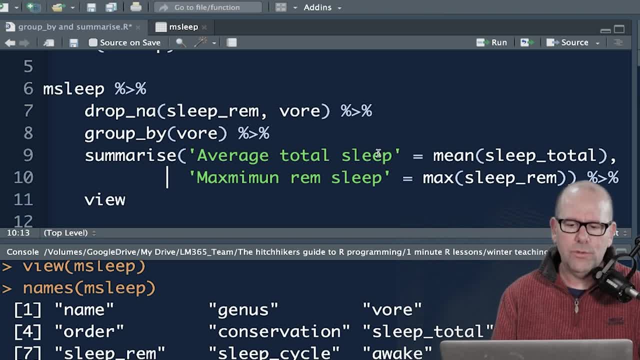 And I just use a little, two little ticks, in which case you can. you don't need to put underscores if you do that. Average total sleep and maximum total REM sleep. So these are the two things. Now. instantly sleep total didn't have any missing values. That's why I didn't include that. 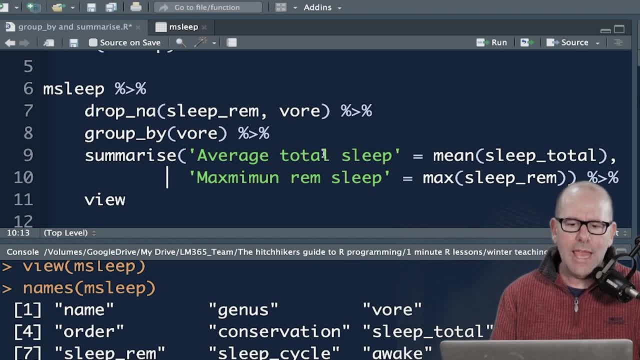 in my dropping in a over there, just so that you know. so average total sleep- that's the new sort of variable that I'm creating as part of my summary- is equal to the function mean, and then the argument in that is which variable you want to have: the average of total sleep. So super duper. 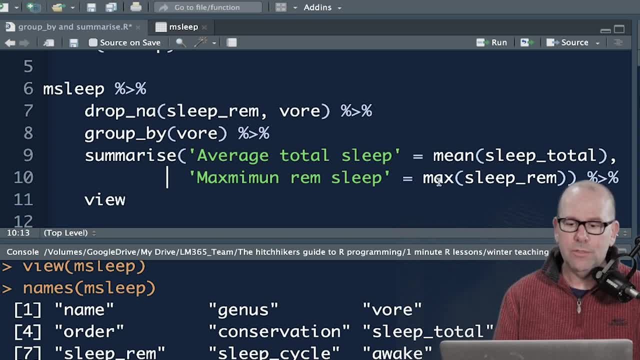 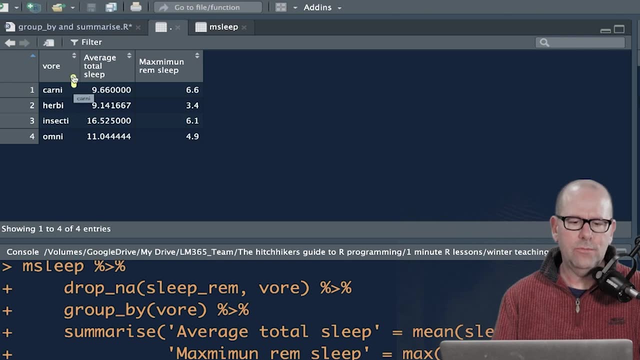 easy, easy peasy, lemon squeezy. then maximum REM sleep is equal to max. that's the function and sleep REM is maximum REM sleep. And then I've said: and then view, So let's look at what that does. Well, so we've grouped by right, so we've grouped by four, So we've got these four groups. 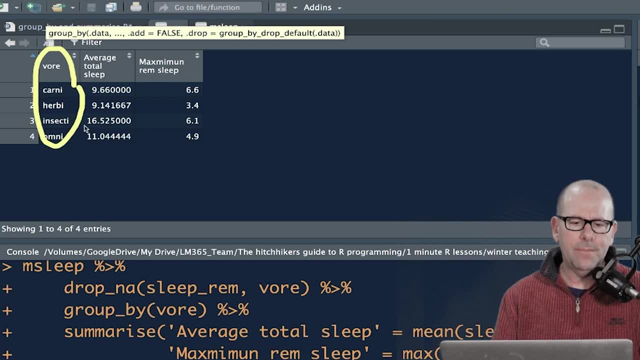 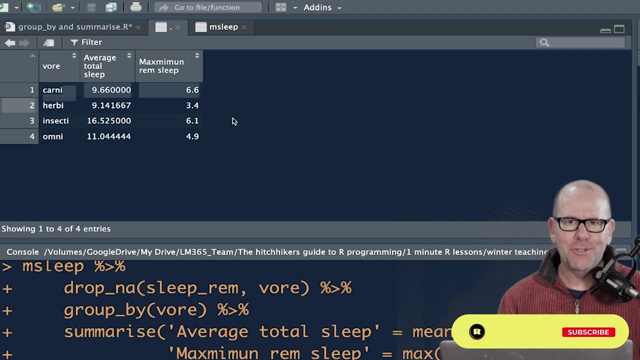 carnivore, herbivore, insectivore and omnivore, And for each of them, for each of these groups, we've calculated the average total sleep and the maximum REM sleep. Can you see that? Okay, super duper, easy Listen. I hope you found that useful. Stay and watch another video, Don't do. 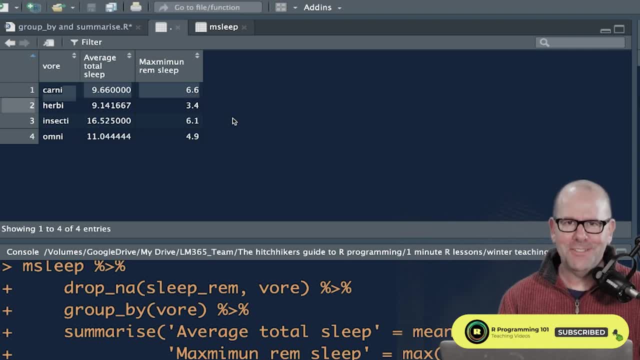 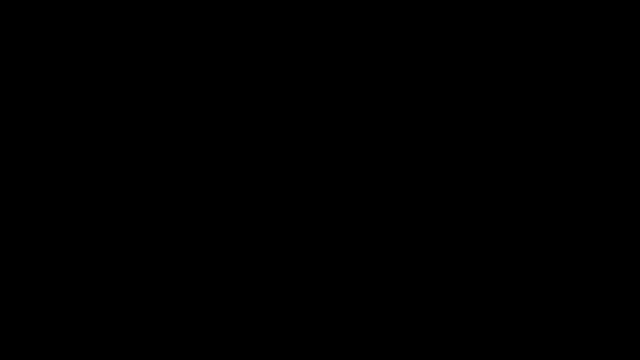 drugs or do this. Don't have a change. It's nice to see you guys Speak to you again soon. Take care Bye.